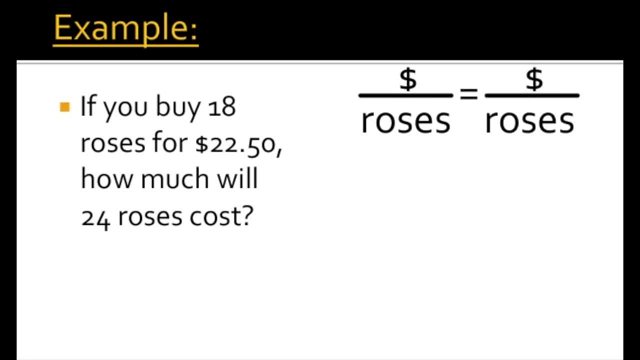 In other words, it's going to have dollars on top and roses on the bottom. So what do we know? We know that we have 18 roses and the 18 roses cost $22.50.. We know that we have 18 roses and the 18 roses cost $22.50.. 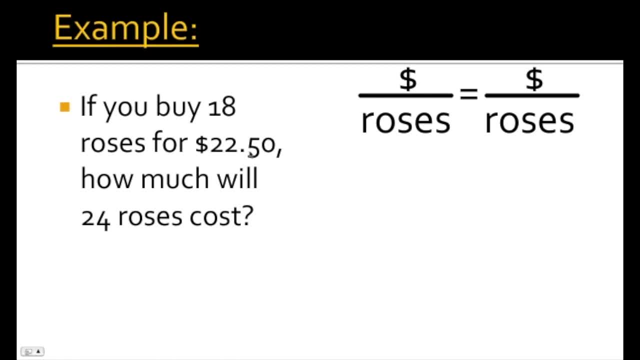 Now for 18 roses. that's going to be on the bottom. we pay $22.50, and that goes on top, So we'll have $22.50 for 18 roses. This is our first ratio. How much do we pay for 18 roses? 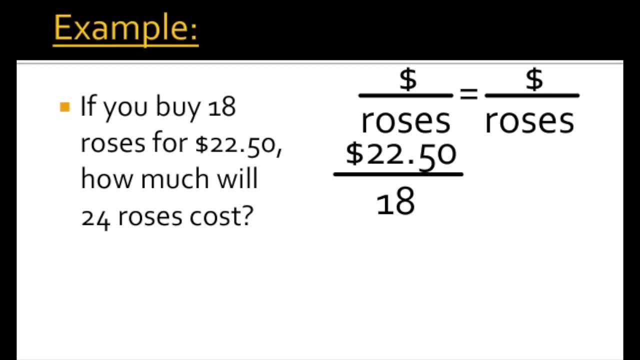 We pay $22.50.. Now the other side will have to set up the same way. But we're missing something. We're trying to find the cost. We have the number of roses. So when we plug our number in, we're going to plug 24 in for the top and the bottom. 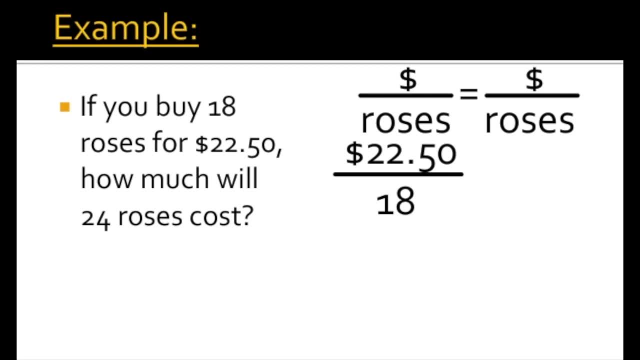 What do you think? Well, we're talking about the roses, so it has to be the bottom, Which means that we're going to have to put a variable in for our numerator, So that's going to be C over 24.. 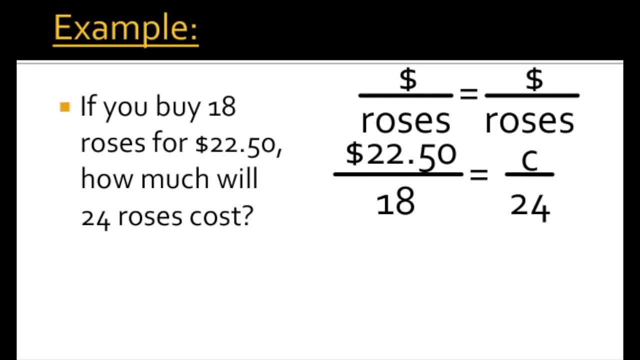 It's also really important to try and choose a variable that actually applies to the problem. For example, here we chose the variable C- C stands for cost- Now that we have our proportions set up- and this is why I said you should know how to solve proportions- 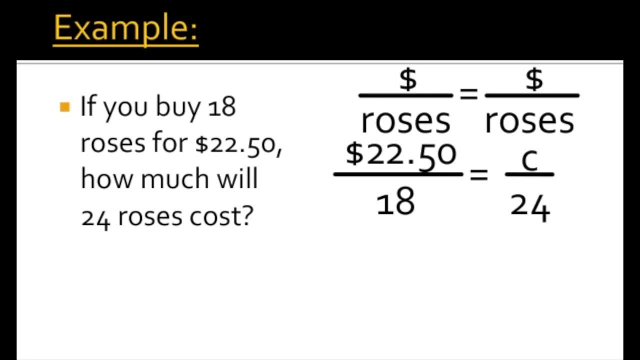 we have to follow the two-step process to solve. The first step is to cross-multiply, So let's do just that. We'll multiply 18 times C and that's pretty straightforward. That's going to be 18C. 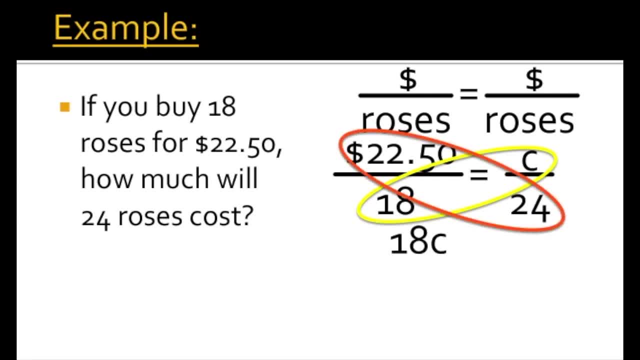 We then multiply 2250 times 24, and that gives us 540.. So now we have: 18C equals 540.. That's step one of solving the proportion. Now step two is to try and get the cost of variable C by itself. 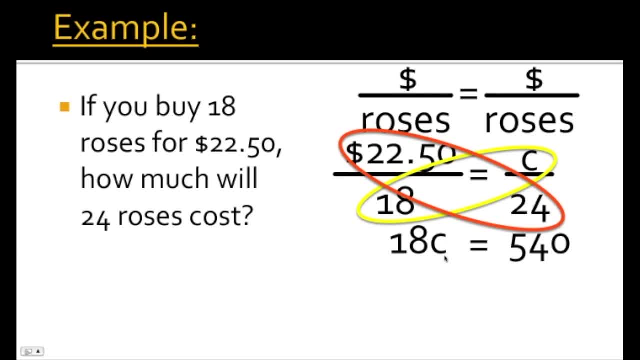 Well, how do we do that? We have to get the variable alone by itself. We get the variable alone by dividing both sides by 18.. When we divide this side by 18, when we divide 18C by 18, what happens is those cancel out. 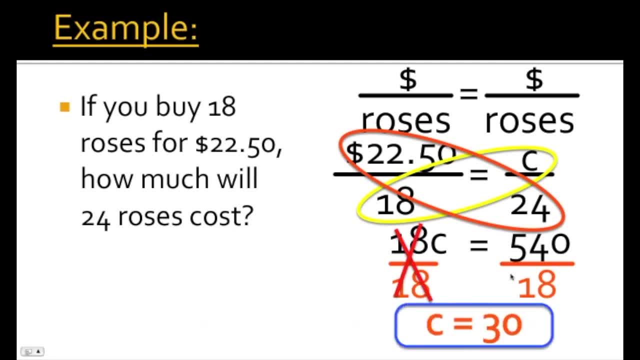 And then we've got 540 divided by 18. That gives us C equals 30. Now it's really important that when you're solving word problems using proportions, you take your answer, the number, and you plug it back into what the question was asking you. 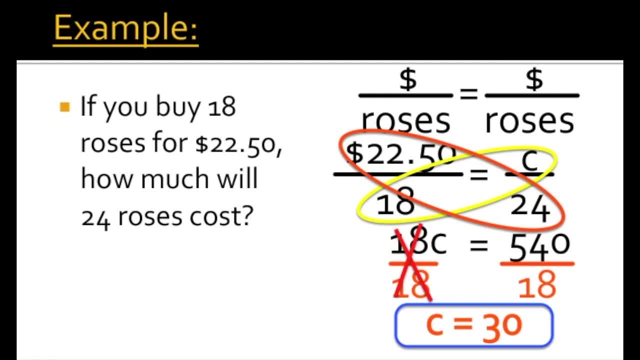 Here we're talking about the cost of 24 roses. What we found was C the cost, So let's plug that back in in terms of the problem. So the cost of 24 roses is $30.. So let's take a look at this example. 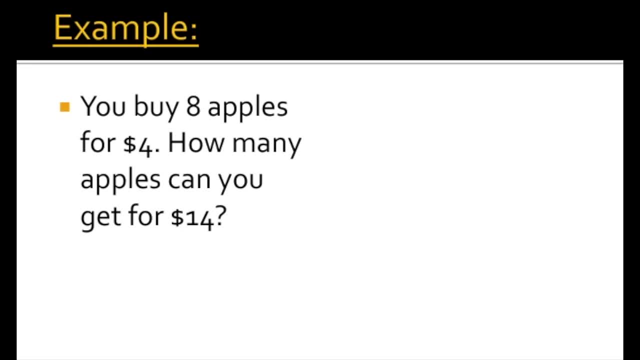 It says you buy eight apples for $4.. How many apples can you get for $14?? Well, we know that we paid $4 for eight apples and we know that we're going to be talking about dollars per apple and that's our first ratio: the cost in dollars for however many apples. 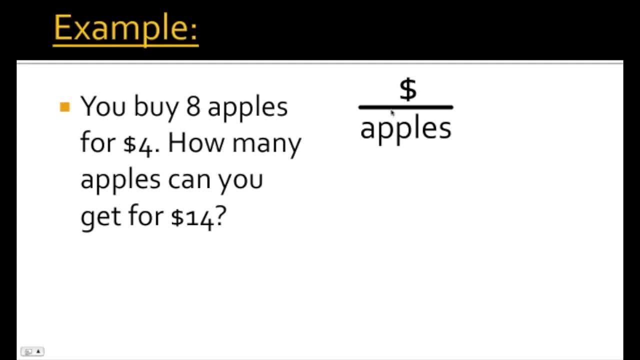 So, since the left side of the proportion is going to be dollars per apples, the right side is going to be set up the same exact way. The other side is also going to be dollars per apples. Well, what do we know? Like we said before, we know that we bought eight apples. 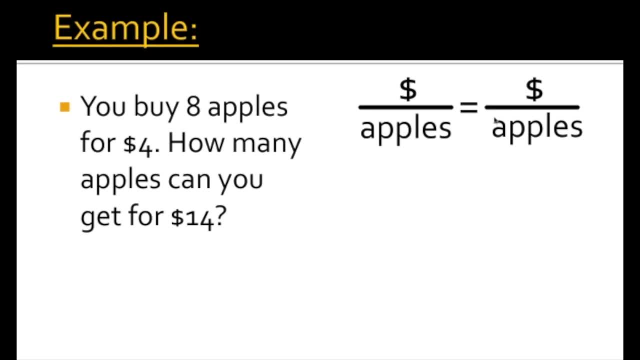 and for those eight apples we paid $4.. So that's our very first ratio: $4 for eight apples. set up exactly the way that we said. we were going to set it up, with the dollars on top and the apples on the bottom. 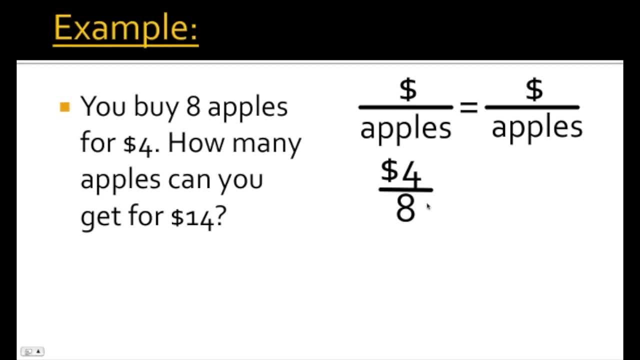 So the other side is going to be set up the same way. but the thing is we're missing something. We're missing information. We're looking for the number of apples. We know that we paid $14. So we know that we paid $14,. 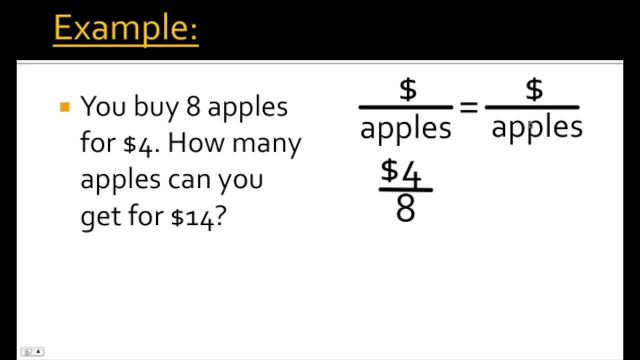 so we'll have the top and the bottom is going to be represented by a variable, So we're going to have it as $14 over A. Now, A is the ideal choice of a variable because we're talking about apples, A for apples. 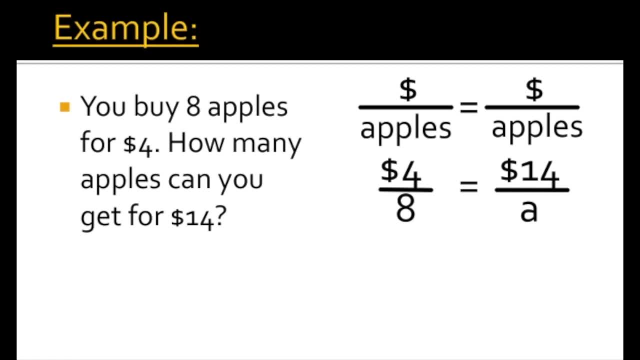 So, now that we have our proportion set up, we just have to solve it mathematically. Now, in order to solve it mathematically, we have to cross, multiply, And the first thing we're going to do is multiply 8 times 14.. 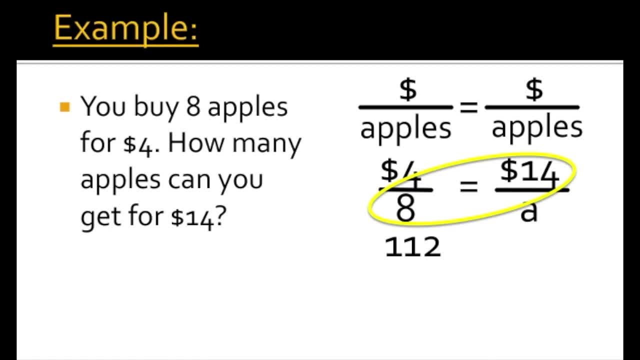 That's going to give us 112.. And then multiply the other ones, which is 4 times A, which gives us 4A. So we have 112 equals 4A. Now, just like any other proportion, we need to try and get the variable A by itself. 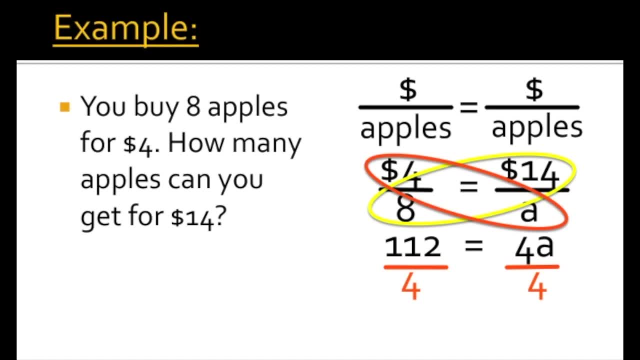 So divide both sides by 4.. This is going to allow us to cancel out the 4s, leaving A by itself, And then we just have 112 divided by 4, and that gives us our answer, which is A is 28.. 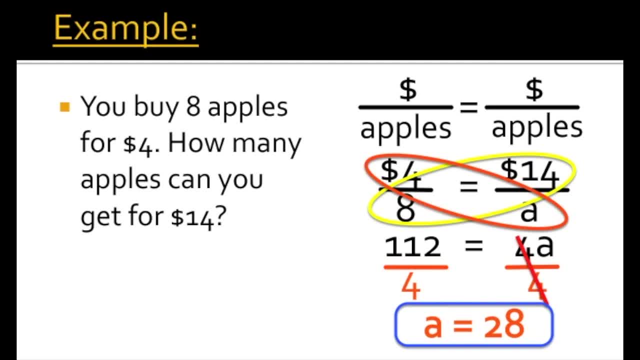 And, just like with the last example, we should take our number and plug it back into the word problem. What were we talking about first place? What was the question we were being asked? We were being asked: how many apples can you get for $14?? 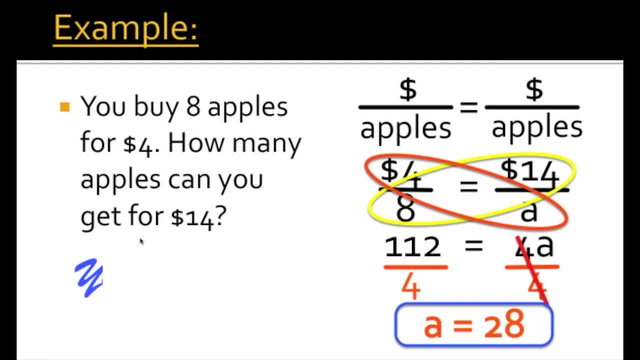 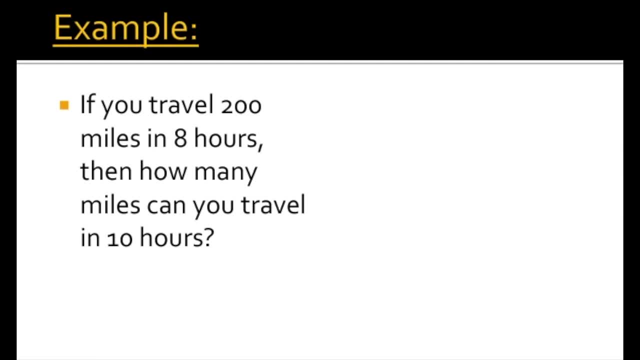 So how many apples can we get for $14?? You can get 28 apples for $14.. Okay, take a look at this example. It says: if you travel 200 miles in 8 hours, then how many miles can you travel in 10 hours? 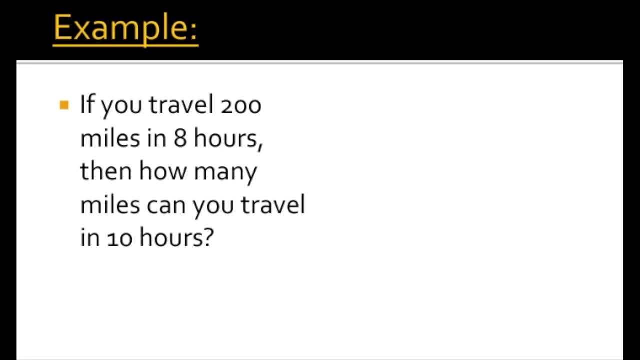 We're talking about traveling in however many miles for a certain number of hours, So our ratio is miles per hour. And now, because the left side of the proportion is set up as miles per hour, we have to make sure that the right side is set up the same exact way. 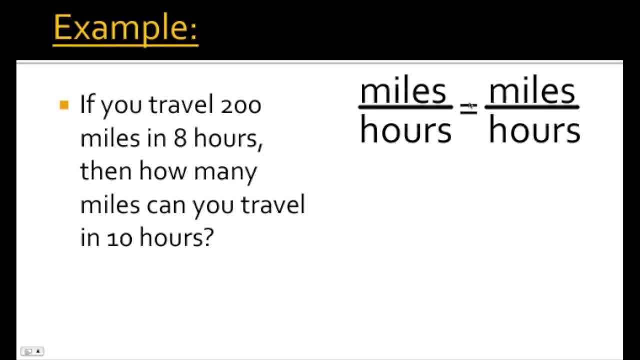 So here we're also going to have miles per hour. Well, what do we know? We know that we can travel 200 miles in 8 hours, So let's set that side up. We'll have 200 miles in 8 hours. 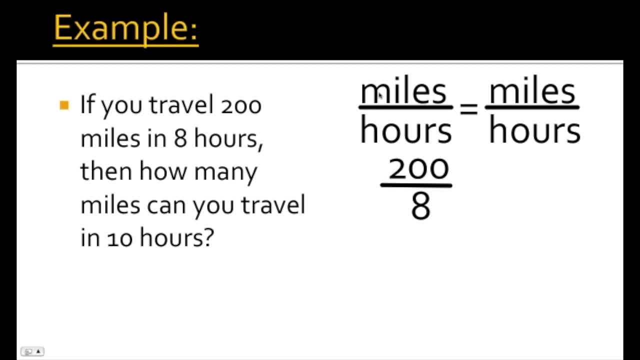 That's going to be 200 over 8, because it's 200 miles. Miles goes on top and we have 8 hours. 8 goes on the bottom. So that's our first ratio. So what exactly are we trying to find? 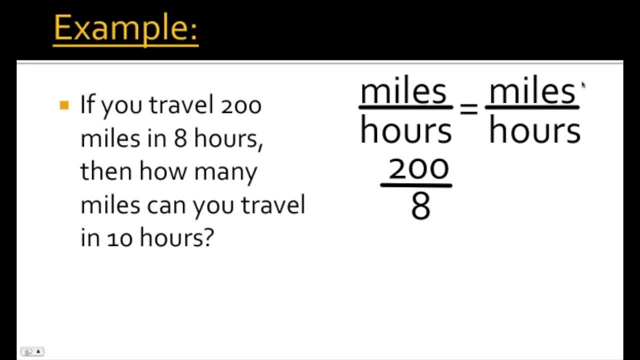 Well, we're trying to find out how many miles we can travel in 10 hours. So what we have is the number of hours. We have the denominator, which is going to be 10.. What we don't have is the number of miles. 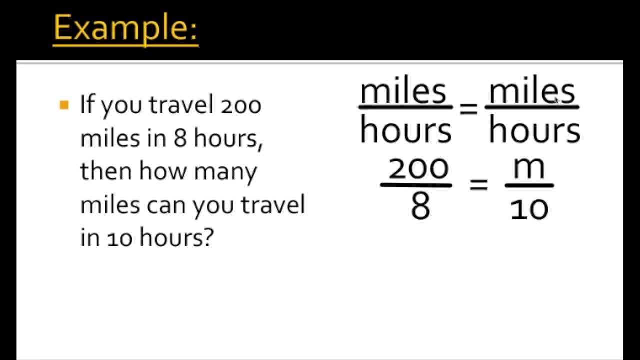 So we'll set this side up as m over 10. And remember, it's always good to choose the best variable for the question. Here, what we're missing is miles, so we're going to actually leave the variable as m. 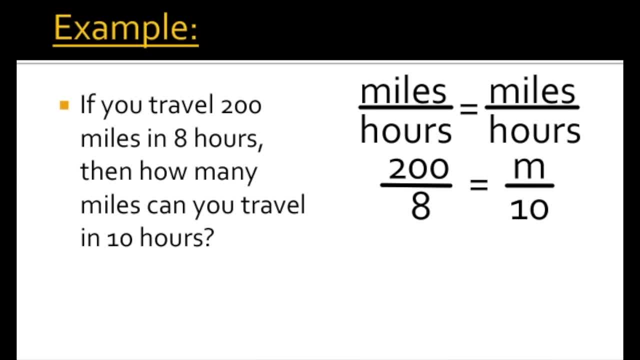 m for miles. So, now that we have our proportion, what do we do next? Well, like we said before, same exact thing as before. we have to solve it mathematically, And there's two steps to doing this. The first is to cross multiply. 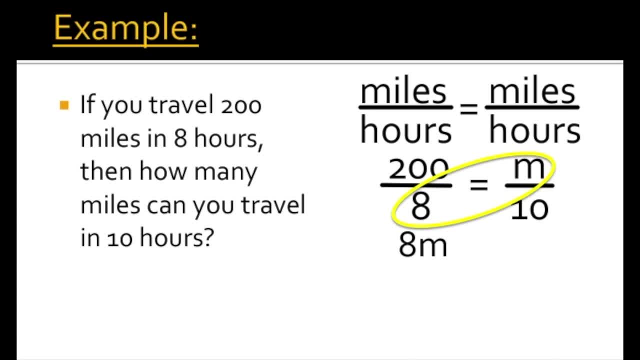 So we're going to multiply 8 times m. That gives us 8m. And then we multiply 200 times 10.. That will give us 2,000.. So we have 8m equals 2,000.. 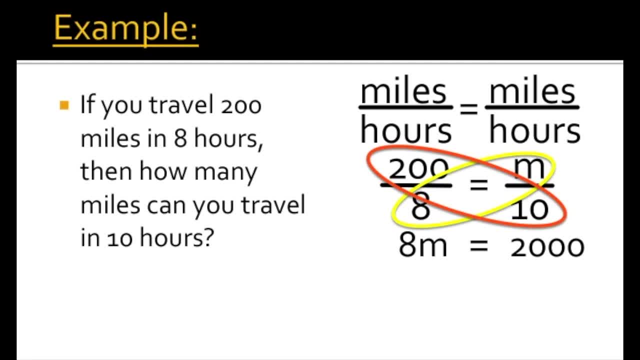 Now the second step is to try to get the variable by itself. We need to divide both sides by 8.. So the 8s are going to cancel. So now I'll have m by itself, the variable m alone. 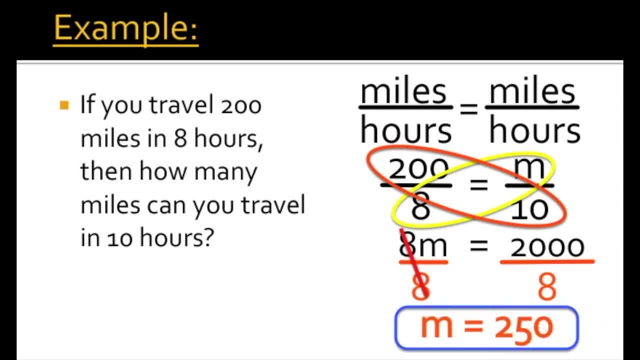 m equals 2,000 divided by 8, which is going to give us 250.. So m equals 250.. And, just like with the last example, it's good to take the answer that we got and plug it back into what we were talking about in our word problem. 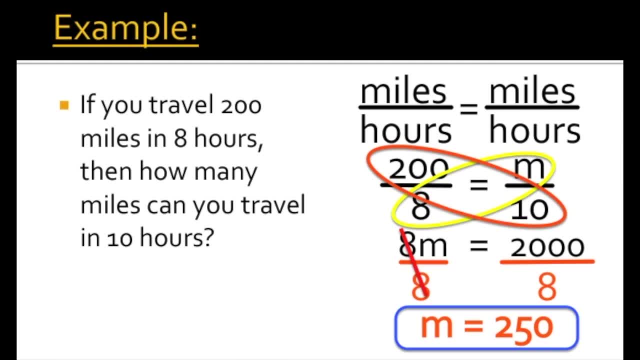 We're talking about miles per hour, traveling a certain number of miles in a certain number of hours. Well, we're saying: how many miles can we travel? How many miles can you travel in 10 hours? Well, we got the answer, as m is 250,. 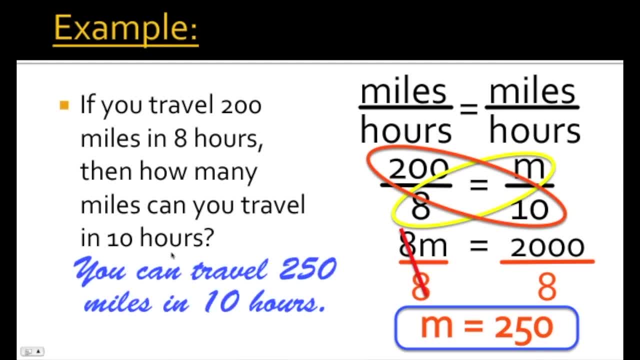 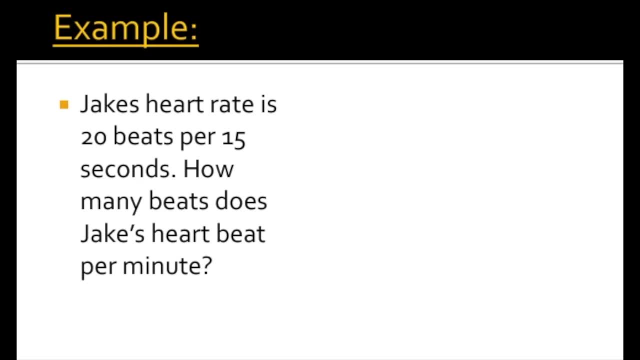 so our answer is: you can travel 250 miles in 10 hours. And for this example, we're saying Jake's heart rate is 20 beats per 15 seconds. How many beats does Jake's heart beat per minute? This one's a little bit difficult. 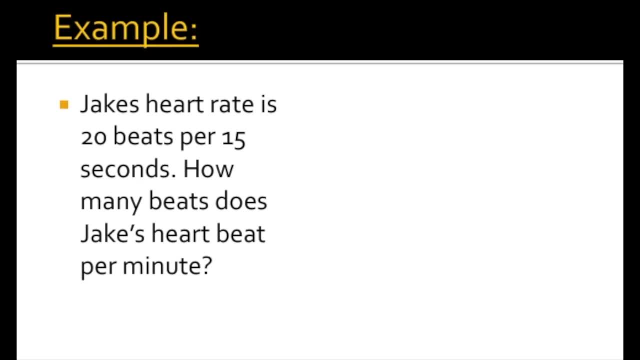 because we don't have the same units in both parts of the question. Here's what I mean. What do we have? We're talking about the number of heart beats that Jake has for a certain number of seconds, So we're talking about beats per second. 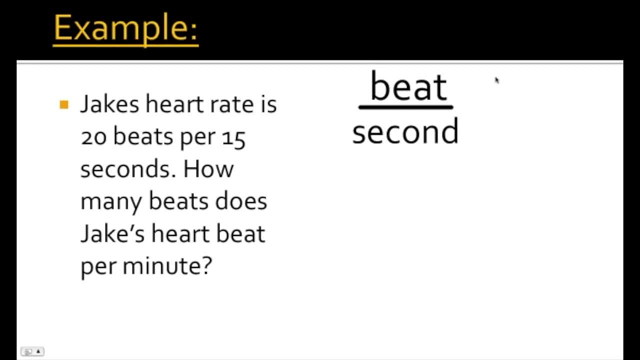 And because the left side of the proportion is beats per second, the right side is also going to have to be beats per second. So what do we know? We know Jake's heart rate is 20 beats per 15 seconds. So the top of our proportion talks about beats. 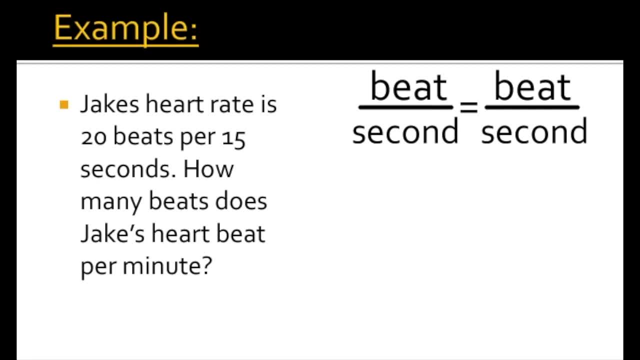 The bottom of our proportion talks about seconds, So we'll plug that in 20 over 15.. So 20 talks about the beats and 15 talks about the number of seconds. Now the right side has to match the left side. 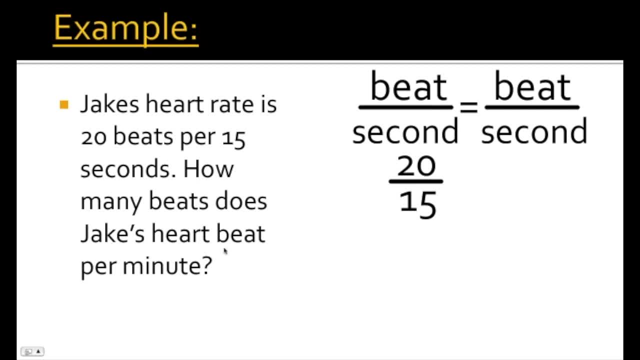 But we're asking: how many beats does Jake's heart beat per minute? Well, it tells us here minute. But what we're talking about in our proportion is the number of seconds. So what are we really looking for If we're talking about the number of beats per minute? 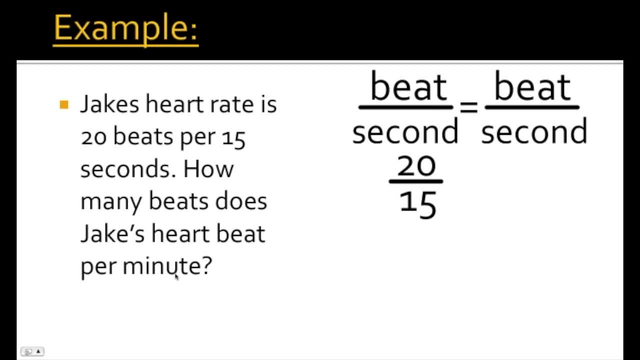 well, how many seconds are in a minute? That would be 60 seconds. So what we're really saying is: how many beats is it for 60 seconds? So let's plug that in. We've got B over 60.. 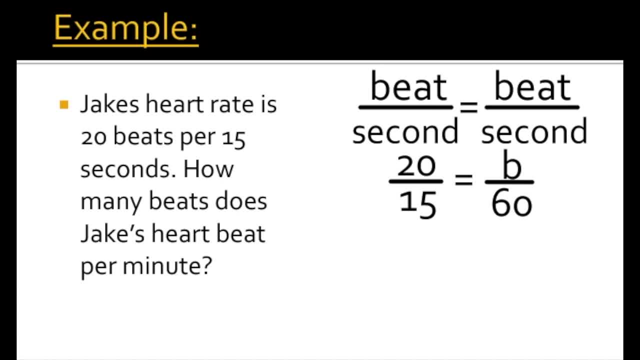 Well, again, why did we put in 60 instead of 1? Because we're talking about one minute. Again, because you have to make sure that the bottoms of your proportions talk about the same thing and use the same units. So now that I have my proportion, 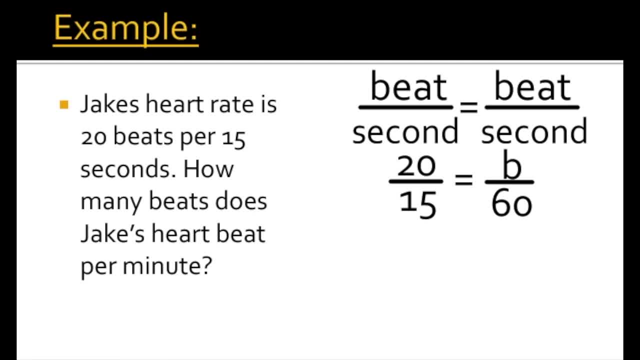 what do I do? I try to solve it mathematically. Remember, there's two steps. The first step is to cross multiply. I've got 15 times B, That's going to give me 15B, And I've got 20 times 60.. 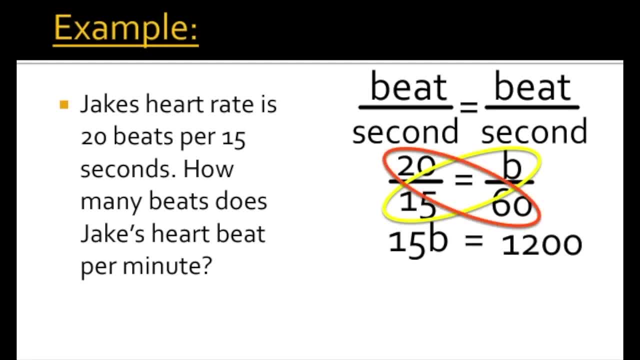 And that's going to give me 1,200.. So now, what do I do? I have to get B by itself. In order to get B by itself, I have to divide both sides by 15.. When I do that, 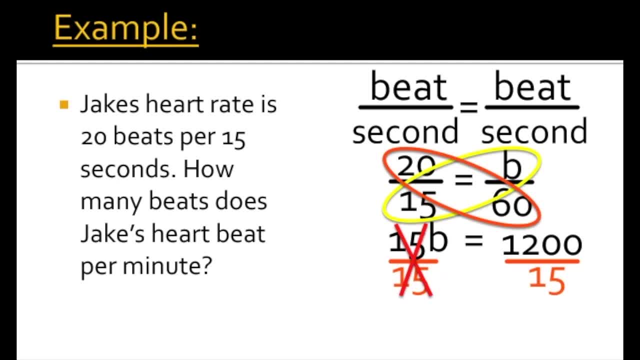 the 15's cancel out, I'm left with 1,200 divided by 15.. Well, what's 1,200 divided by 15?? That's going to give me 80. So B equals 80. Again, let's relate that back to the word problem. 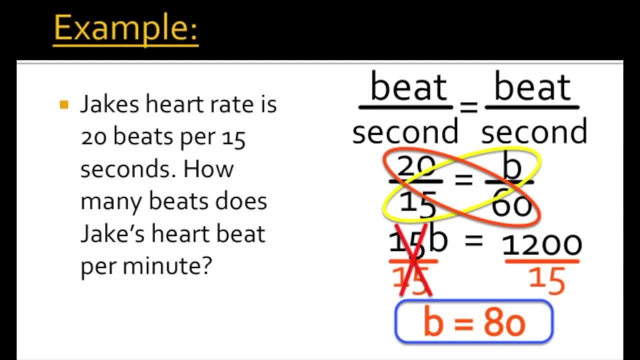 In the word problem we're asking: how many beats does Jacob have and how many beats does Jake's heart beat per minute? Well, since B is 80, what we're really saying is: Jake's heart rate is 80 beats per minute. 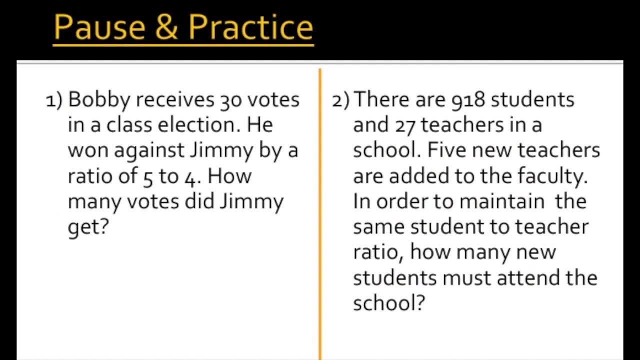 So here's your pause and practice. Just pause and practice. When you're done, unpause the video. After a 3-2-1 countdown, your answer will be displayed. Go, Okay. so, since there's only two questions, 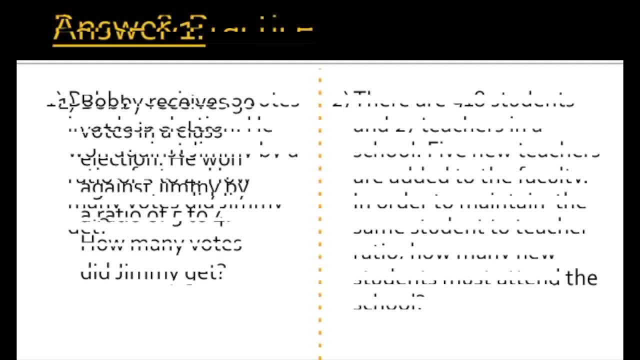 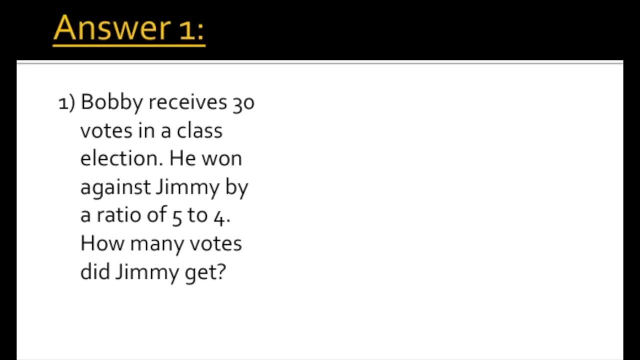 let's go over these one at a time, Starting with number one. Number one says Bobby receives 30 votes. in a class election, He won against Jimmy by a ratio of 5 to 4.. How many votes did Jimmy get? So we know that Bobby receives 30 votes. 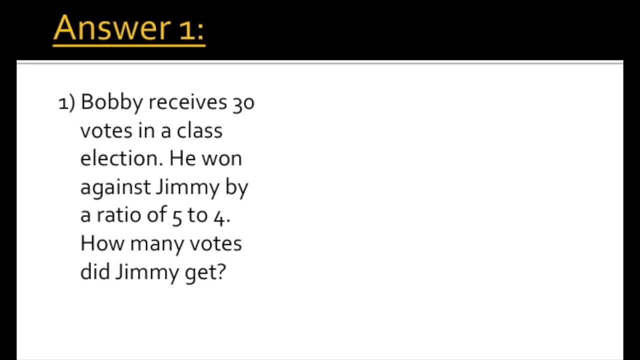 in that class election. What we're talking about is the ratio of Bobby's votes to the number of Jimmy's votes. So let's set that side of the proportion up, So it's going to be Bobby's votes over Jimmy's votes. Now, because this side 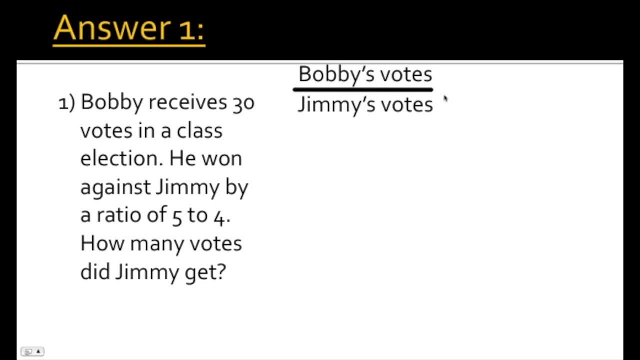 of the proportion is Bobby's votes over Jimmy's votes. we have to make sure the other side of the proportion looks exactly the same, So we'll set that up as Bobby's votes over Jimmy's votes. Now, what we know about Bobby's votes is that there's 30 of them. 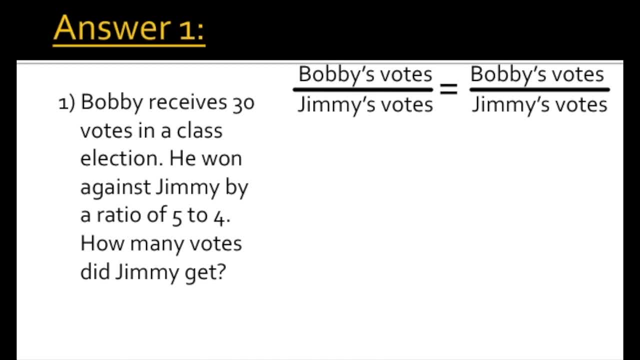 So he got 30 votes. What do we know about Jimmy's votes? We don't know how many votes Jimmy's received yet, and that's what we're trying to find. So when we set this side of the proportion up, we know. 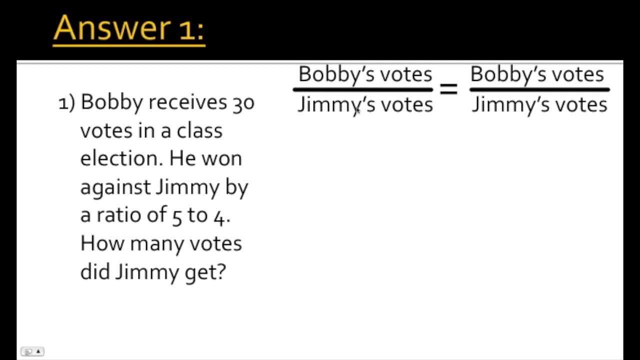 Bobby's got 30 votes and Jimmy we don't know yet. So what's the best variable to use? J for Jimmy? So we've got 30 over J equals. well, what? What other information do we have? 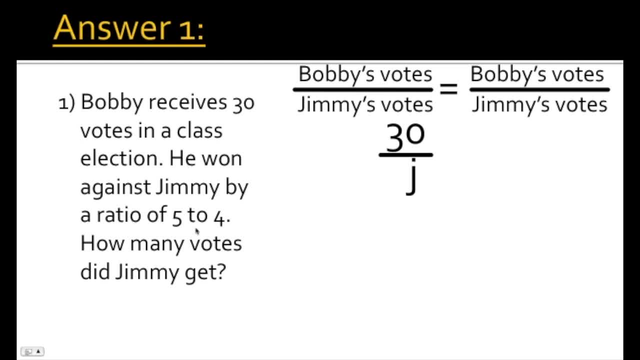 We do have the information that says that he won against Jimmy by a ratio of 5 to 4.. So 5 is going to represent the number of votes that Bobby got and 4 is going to represent the number of votes that Jimmy got. 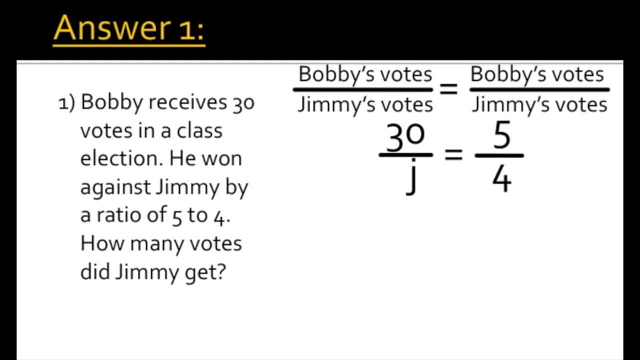 So let's plug those in. So now we've got 30 over J, equals 5 over 4.. We have our proportion set up and all we need to do is solve for J. Well, how do we do that? Remember, there's two steps. 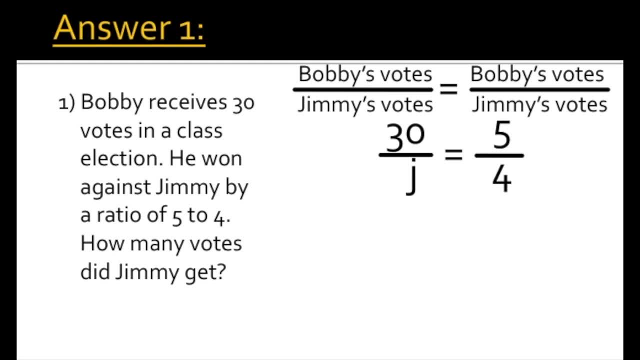 to solving proportions. Step one is to cross multiply. so let's do that. We've got 5 times J, that gives us 5 J. and we've got 30 times 4, that gives us 120.. How do we get J alone? 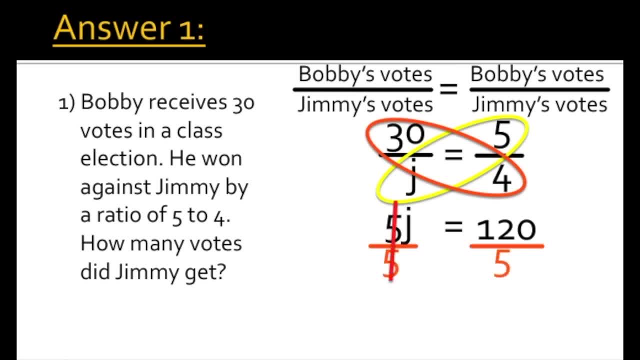 Well, we divide both sides by 5, the 5's cancel and J equals 24.. Now let's plug that back into what we were talking about. What are we being asked in the question? We're being asked how many votes. 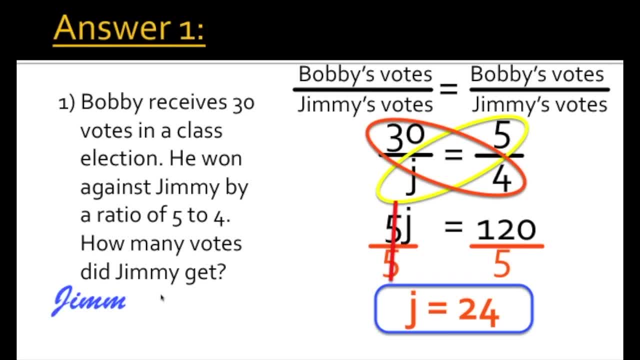 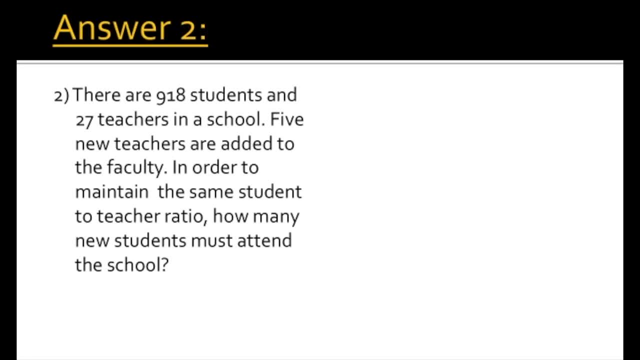 did Jimmy get? Well, we said J equals 24.. Therefore, Jimmy received 24 votes In this one. there are 918 students and 27 teachers in a school. 5 new teachers are added to the faculty In order to maintain. 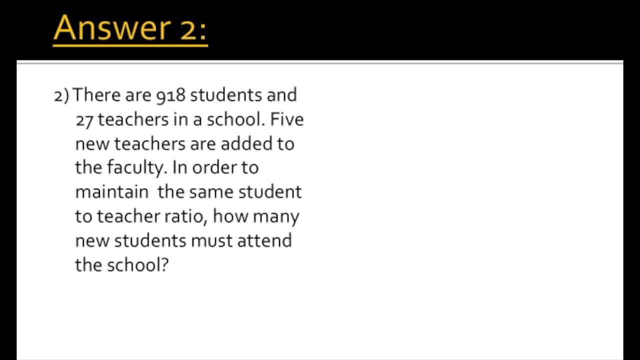 the same student to teacher ratio, how many new students must attend the school? Well, how do we set this proportion up? What are we talking about in the question? We're talking about the ratio of students to teachers. Okay, The top of our ratio. 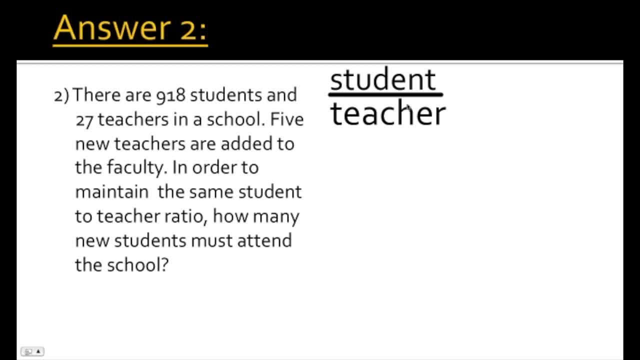 talks about students and the bottom talks about teachers. Therefore, the other side of our proportion should be the same thing: Students to teacher. Now, how many students do we have in the school? We said we had 918 students, And how many teachers? 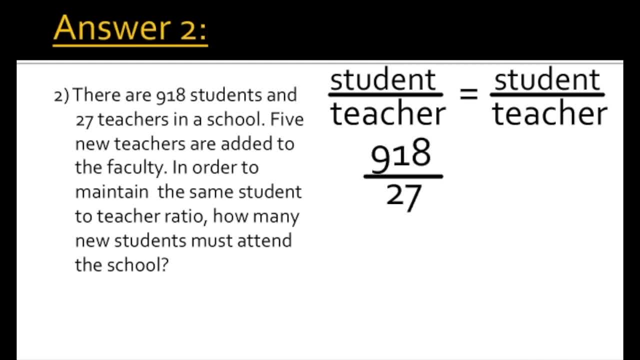 27.. So that information we plug into the first side, to the left side of our proportion. So the ratio of students to teachers is 918 to 27.. Well, what are we trying to do? We're trying to see how we can maintain. 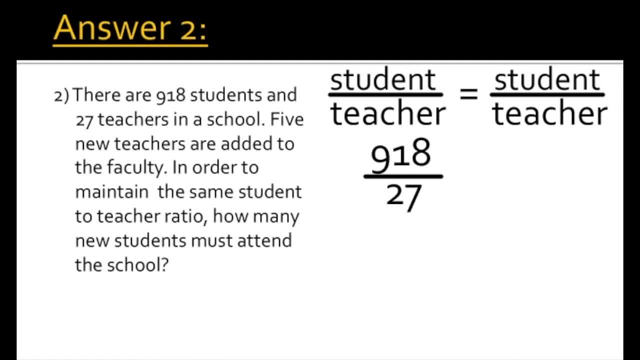 the same ratio by adding a certain number of students. It says 5 new teachers are added. So for every 5 teachers, how many students are there? Well, let's try and figure that out. The left side of our proportion says 918 over. 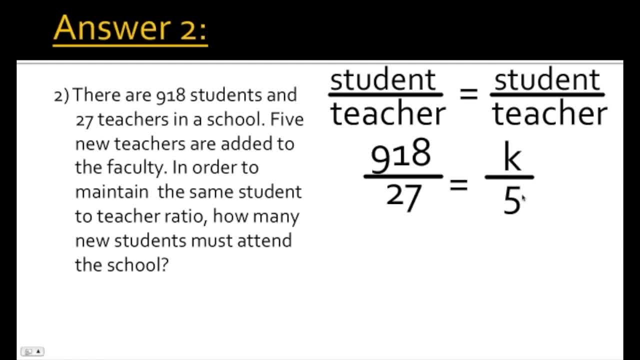 27.. The right side is k over 5.. Normally I select a variable that's easier to relate to the question, but I try to stay away from using s as a variable because s kind of looks like the number 5.. So I chose.